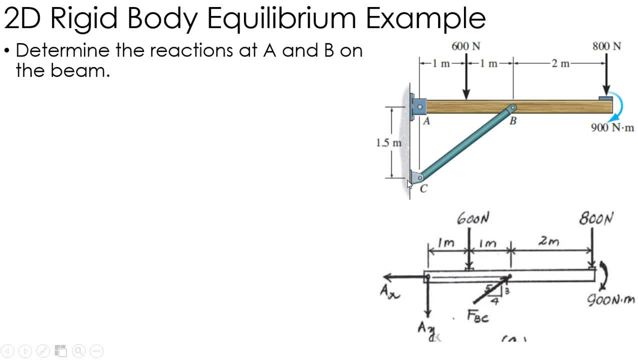 Okay, Meaning that the force has to be equal, opposite and collinear. That means the force has got to be directed along the line of B to C, Okay, Which actually is a 3, 4, 5. Triangle or a 1.5, 2, 2.5 triangle. So I know that that force is in that direction, So I draw that in there. Again, if I have it pushing up, it might be pulling on it. I'll just get a negative answer if I'm wrong. But recognizing that this is a two-force member, therefore the force is directed between those two points, is important in drawing my free body diagram And that takes care of all of the moments and forces. 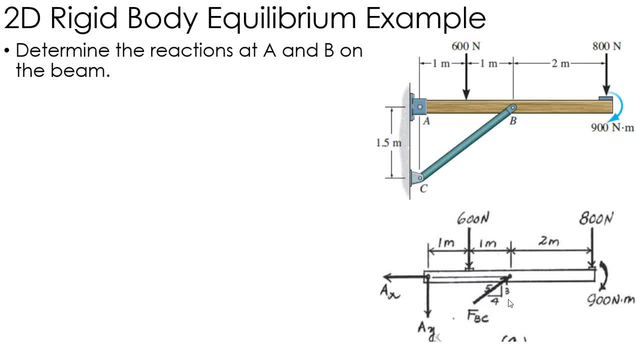 Now I'm actually going to start with my moment. equilibrium equation. Right, I have three equilibrium equations: Some of the forces in the X and Y and then the sum of the moments. I'm actually going to sum the moments about point A And the reason I'm going to sum them- because I can choose any point to sum the moments about. The reason I'm going to choose point A is because I have both AX and AY at that point. So when summing the moments of all of these forces in this couple moment, Okay, The moment of AX and AY. 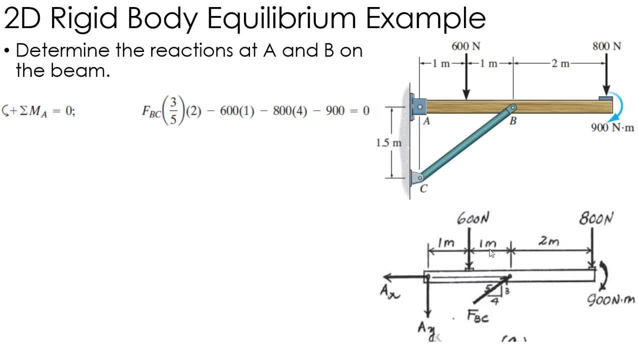 are zero, So they do not show up in the equation. The only unknown that's going to show up in this equation, the only force about point A, the only unknown force about point A, is going to be FBC, Because these two pass right through. They have zero moment about point A. Okay, So FBC, the horizontal component goes right through point A. So I'm really only concerned about the vertical component, which is three-fifths FBC, And that's at a distance two meters away. So I'm 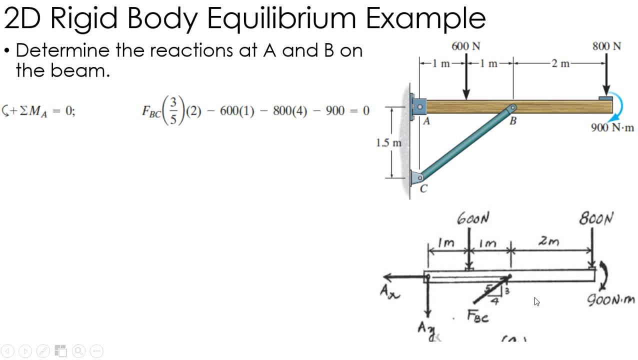 going to get two, three-fifths FBC. That's the moment of this force. about point A: Again, AX and AY have no moment, Okay. Then I have 600 one meter away, And that's actually creating a negative moment, A clockwise moment. I have 800 four meters away, creating a negative moment. Okay. So those are all of my forces. 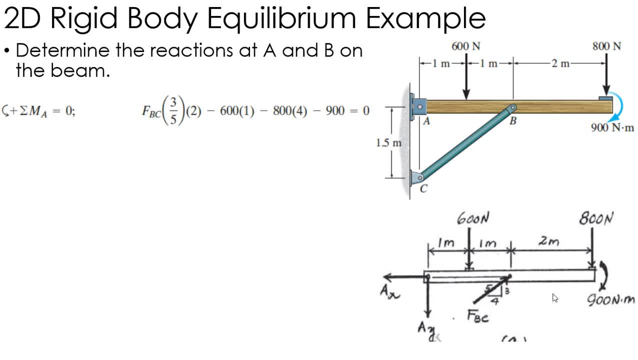 Okay, The moments of all the forces. I also have this 900 newton meter couple moment And it's a negative couple moment, It's a clockwise couple moment. Now, the location of that's not interested, So you'll note, or not important, excuse me. So you'll note that I don't multiply that times any distance, Right, That couple moment is a free vector. It acts basically everywhere on the beam, So I just throw that in there Minus 900.. The location's not important. 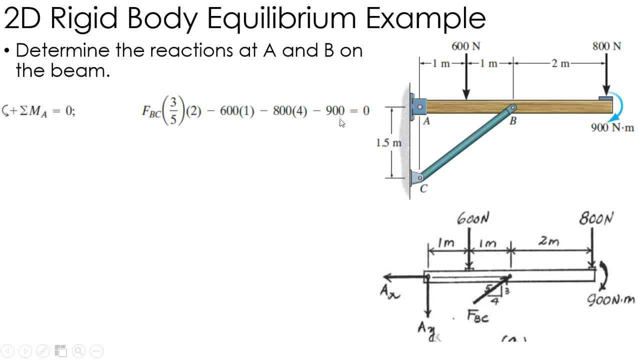 I don't multiply times four or anything like that, I just put in 900.. As opposed to the forces which their location is important, I'm taking 800 newtons times four meters, or 600 times one meter, or three-fifths FBC times two meters. Okay, So this is my moment equation And now summing the moments about A, again, the only unknown is FBC. here The AX and AY do not show up, So I can solve for FBC and I find that it's 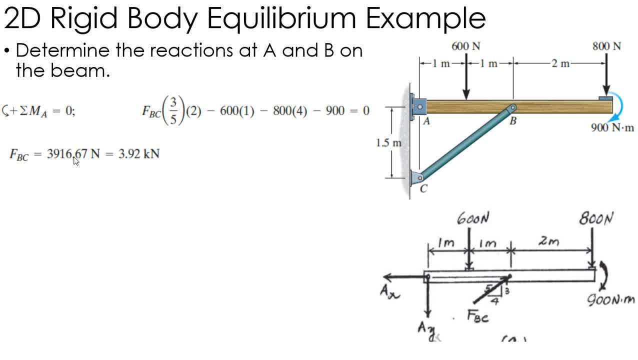 3.92 kilonewtons or 3,916 or 17 newtons, Okay, So choosing that point. to take a moment about being A, I can directly solve for FBC. Now I'm left with two unknowns, AX and AY, that I will put into some of the forces in the X and some of the forces in the Y direction. So in the X directions I have the four-fifths FBC, the horizontal. 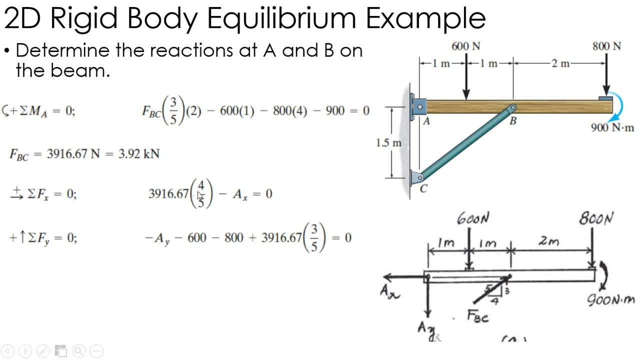 direction. So this is FBC, which I just solved, four-fifths and minus AX, AX being the only other force in the X direction. So I can directly solve AX from that equation. My Y direction, I have minus AY, minus 600,, minus 800, and then three-fifths FBC. Okay, Again, the couple moments aren't going to show up anywhere in the force equations because it's not a force, it's a moment, Okay. 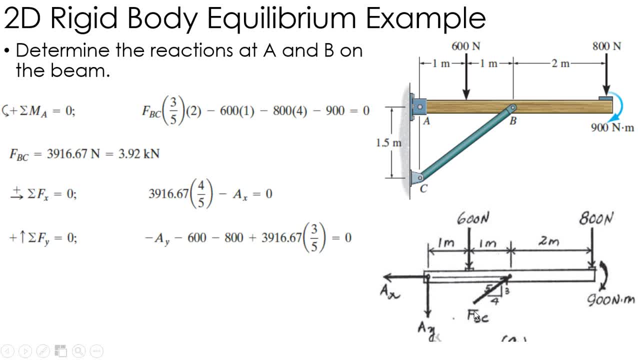 So in the Y direction, minus AY, minus 600,, minus 800, plus three-fifths FBC. Again, the only unknown in this equation is AY, So I can solve these two equations directly. I find AX equal to 3.13 kilonewtons and AY equal to 950 kilonewtons.